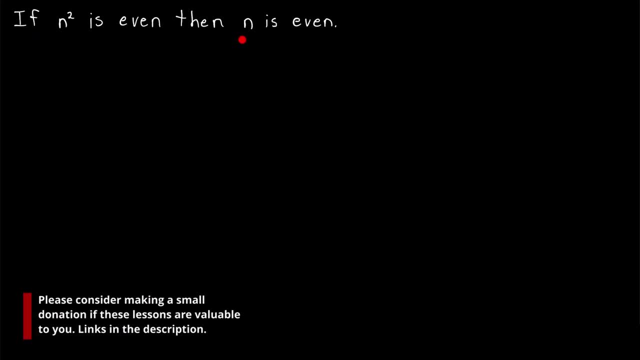 If n squared is even, then n is even. This makes for a great proof by contrapositive. so that's what we're going to do in today's Wrath of Math lesson. What we have here is a pretty standard conditional statement. If p, then q, And we could prove this directly. You might do. 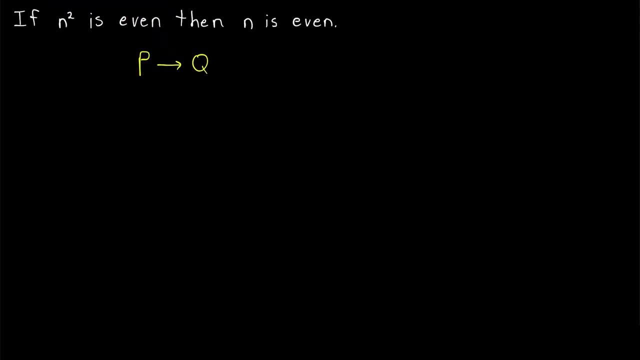 something like say: okay, we know that n squared is even. That means n squared equals 2 times k for some integer k. Then you may think doing something simple like just taking the square root of both sides gives us n equals the square root of 2k, And that doesn't seem tremendously. 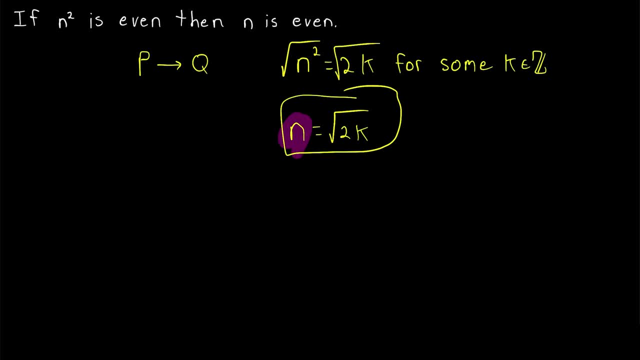 useful for proving that n is even, which is what might make you think to try something else like a proof by contrapositive. But if you think about it a little bit more, you might think. well, n squared being even means that. 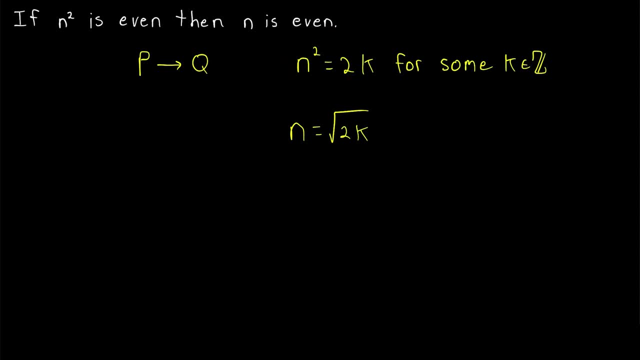 2 is one of its prime factors, And you can't create a prime factor of 2 by squaring a number, which means the prime factor of 2 must have already existed in just n. n must have had a prime factor of 2, which means that it has to be even in order for n squared to have a factor of 2.. 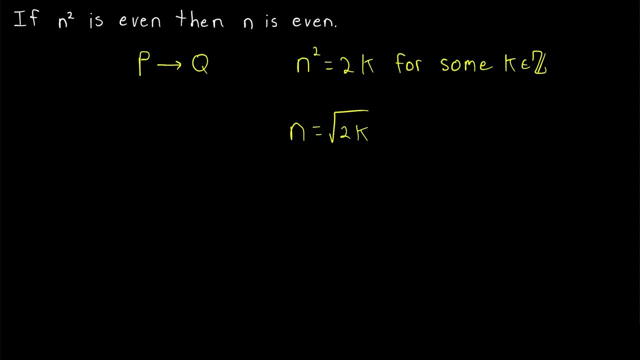 And so you could write that up a little more formally and be done. But that certainly takes a little bit more creativity than a simple contrapositive proof. Doing this by contrapositive is super easy. Remember the contrapositive of an if p, then q statement is: if not q, then not p. 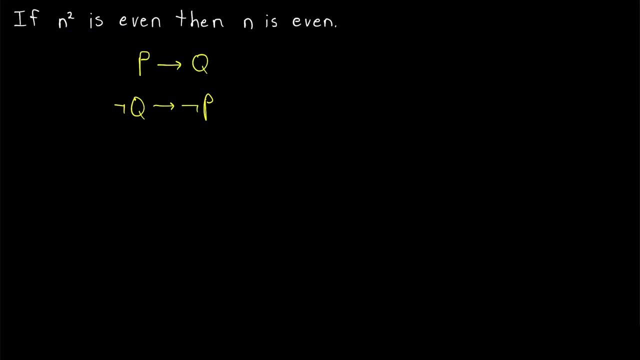 What's the contrapositive of this statement here? Well, originally we had: if p, n squared, is even, then q, n is even. So the contrapositive is: if not, q, which is if n is not even. 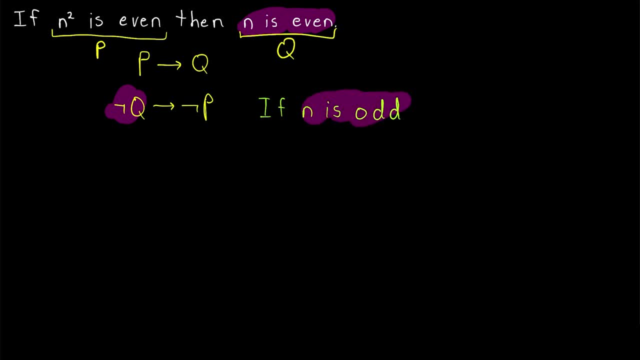 meaning that n is odd, since we're talking about integers here. So if it's not even, it's got to be odd. So if n is odd, then not p. p is n squared is even So not p is n squared. 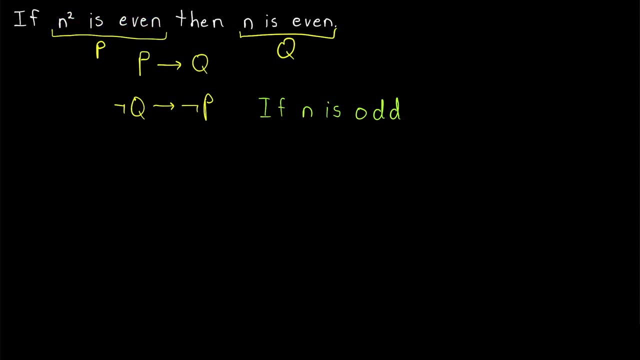 is not even Again, since we're talking about integers, that means that n squared is odd. Of course, if n could be any real number, then it might be something like 2.5, which isn't even or odd. So here is our contrapositive Again. all we had to do was flip the order of the statements. 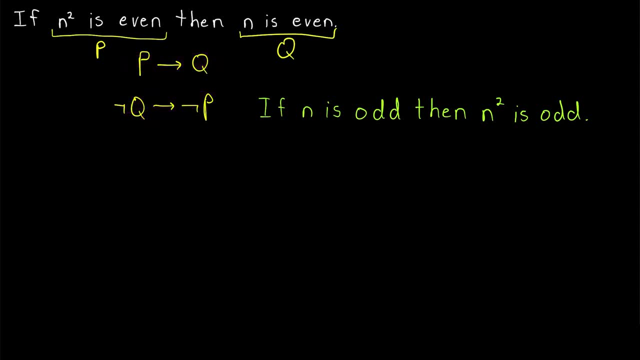 and negate them. So instead of assuming that n? squared is even, we're concluding that n? squared is odd. And instead of concluding that n is even, we're concluding that n squared is odd. If n is even, we're assuming that n is odd. The whole point of the contrapositive, remember. 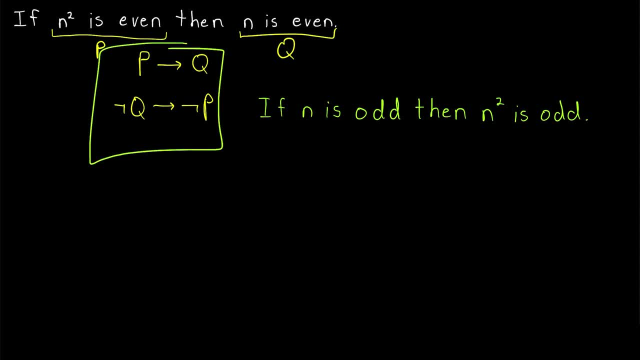 is that these two things are equivalent, So we can prove either one we want. They are the same. So to prove the original statement, all we have to do is prove that if n is odd, then n squared is odd, because proving the contrapositive is just as good. 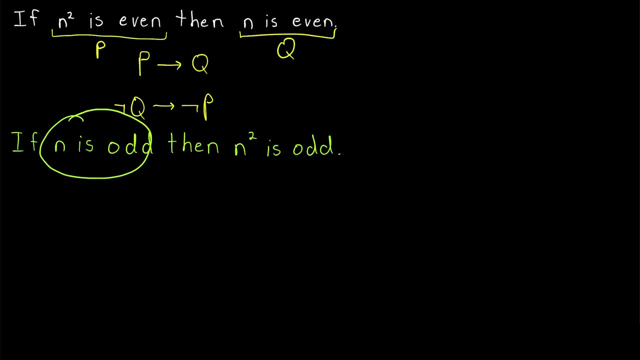 This ends up working pretty nicely, because if n is odd, then, by definition of an odd number, n equals 2k plus 1 for some integer k. And now, instead of trying to take a square root like we were doing before, 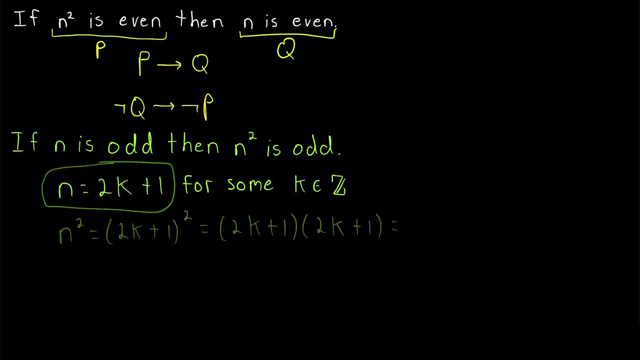 we just have to square n, which is a lot easier. n equals 2k plus 1, so n squared equals 2k plus 1, squared which is 2k plus 1 times 2k plus 1.. That's going to give us 4k squared plus 2k. 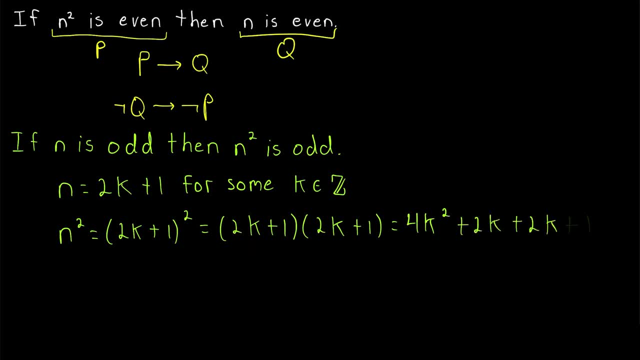 plus another 2k and plus 1.. Then, combining like terms, this is equal to 4k squared plus 4k plus 1.. Remember, this is n squared, which we are trying to show is odd. To show this is odd, we need to show that it's one more than a multiple of two. 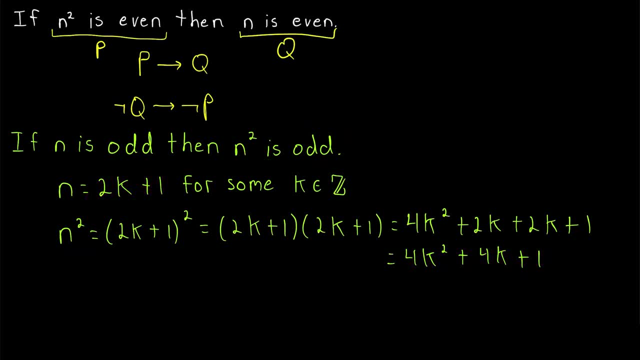 since that's the definition of odd. And well, we have a plus 1 here. we have two terms that have a factor of 2, so all we have to do is take a 2 out of these first two terms. Factoring a 2 out of those first two terms will give us 2 times in parentheses. 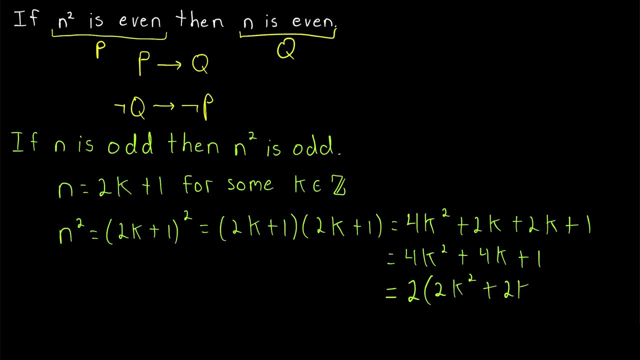 2k squared plus 2k, and then we still have our plus 1 at the end. Notice how, if you distributed the 2 through these parentheses, we'd get what we originally had: 4k squared and 4k, and then our plus 1.. 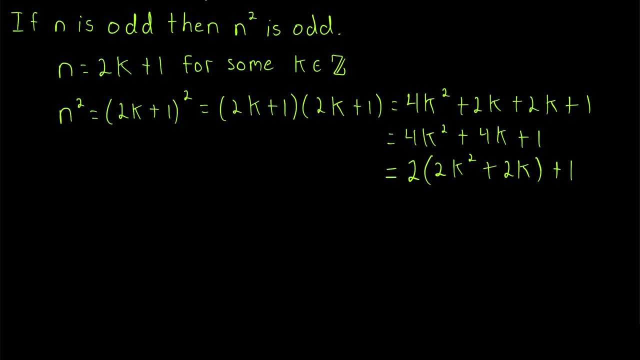 The last thing we need to do is to get the 2 out of these first two terms. The last thing you might point out, especially if this is one of your first proofs, is that this here is an integer. We know this is an integer by closure, because k is an integer. 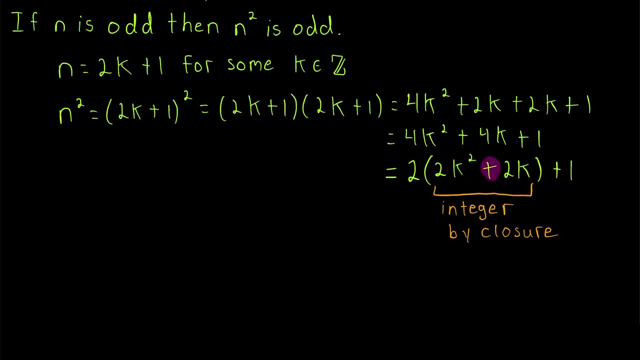 So squaring it, multiplying it by 2, and adding it to 2k, that's just going to give us another integer, because the integers are closed under addition and multiplication. Since this is an integer, we've shown that n squared is. 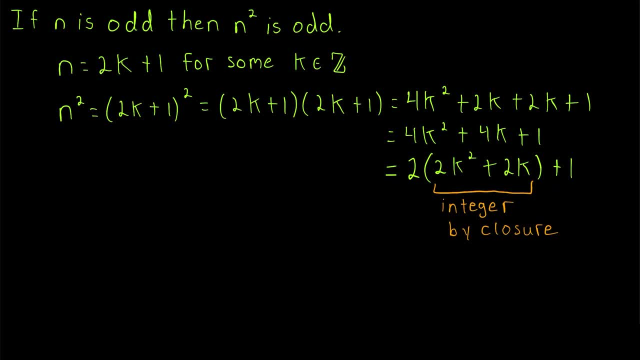 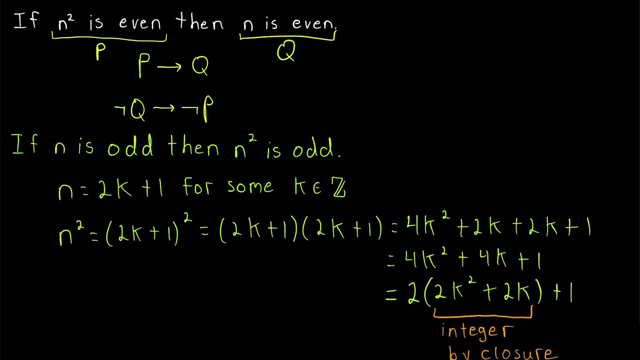 2 times an integer plus 1, which means, by definition, n squared is odd. So we have proven that if n is odd, then n squared is odd, and so, since contrapositives are equivalent to the original statements, we've proven that if n squared is even, then n is even. And take a second to make sure you understand that at a 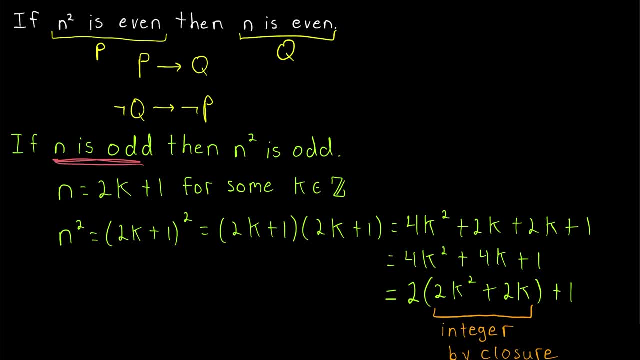 conceptual level, We proved that n being odd forces n squared to be odd. So obviously n squared being even forces n to be even, because if n was odd, well we just proved that n squared would have been odd, so we wouldn't be able to have n squared being even. 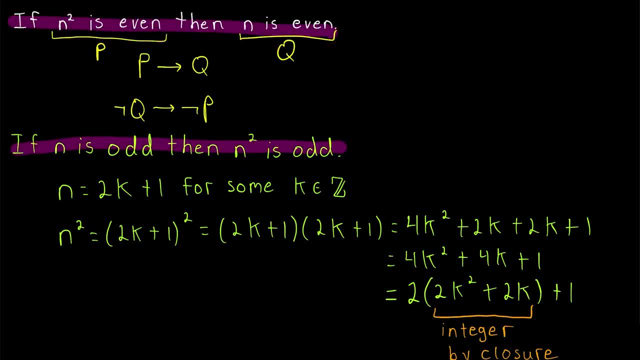 These two statements are equivalent, so the contrapositive is a pretty beautiful thing. Sometimes it's more obvious how to prove the contrapositive of a statement. Other times the original statement you're considering is easier to prove, but the contrapositive. 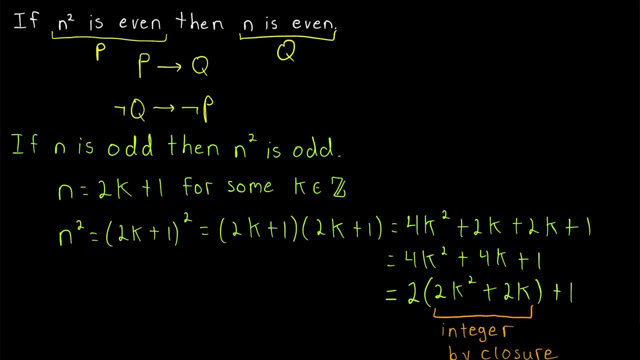 is actually a more useful result going forward. So, with that in mind, not only do you have two options when proving a statement like this, to prove it or its contrapositive, but once you've proven either one, you've proven both of them, and sometimes that's really useful. Subtitles by the Amaraorg community.